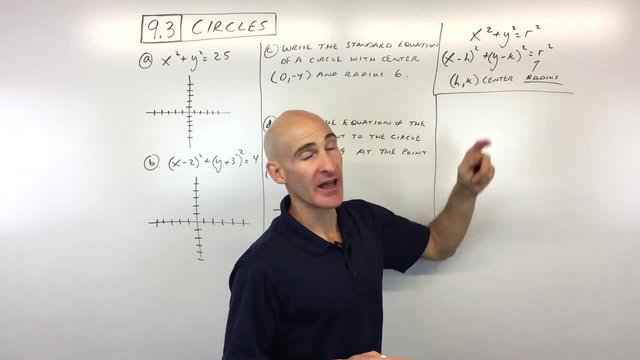 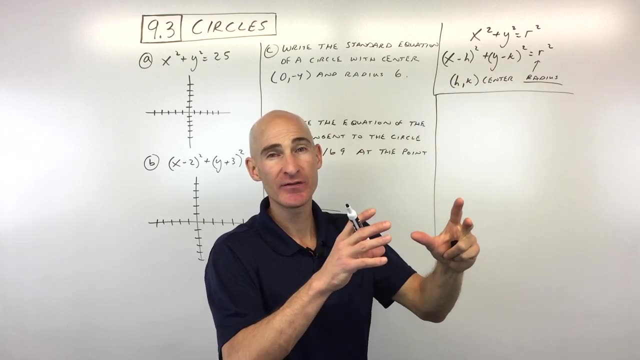 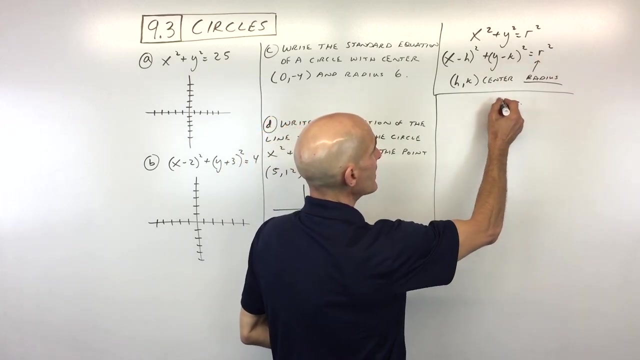 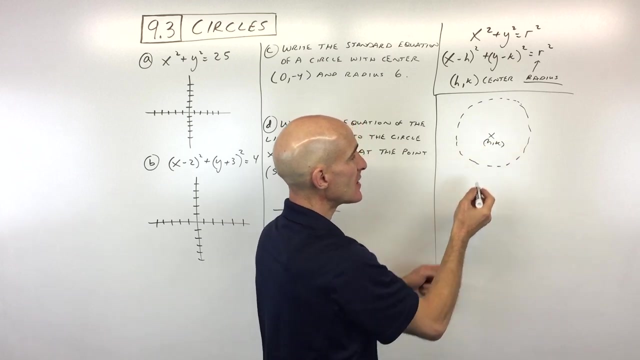 It's just that it's been shifted: hk. So basically this is shifting left and right, this is shifting up and down. hk is the center of the circle, so it's being shifted, And then r, of course, again, is the radius. So what exactly is a circle? Well, a circle is a set of all points that are equidistant from a given point, which is called the center. We're going to call the coordinates of the center hk, So that's the center point, right there. Now, if you take a point on the circle, 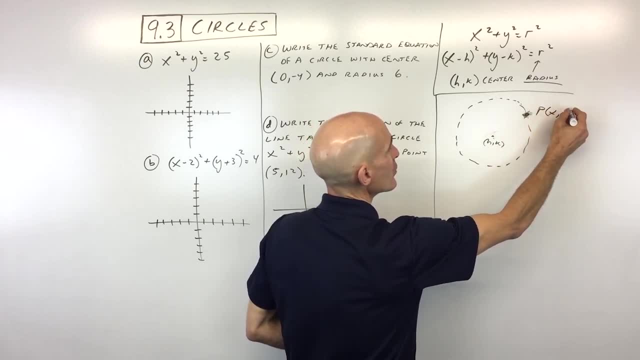 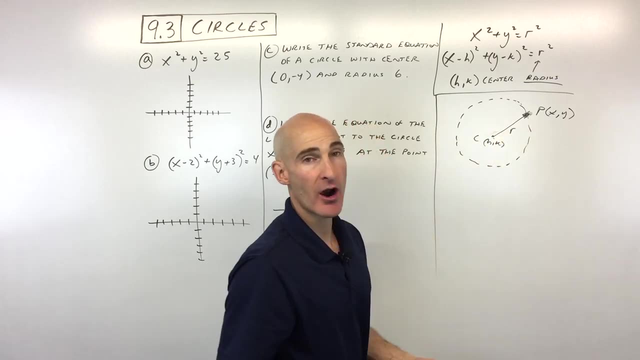 let's just make a point on the circle like that. Let's call that p and the coordinates of that point we're going to call xy, But the distance from the center to that point on the circle, that distance, we're going to call r, the radius, So you can see all these points. 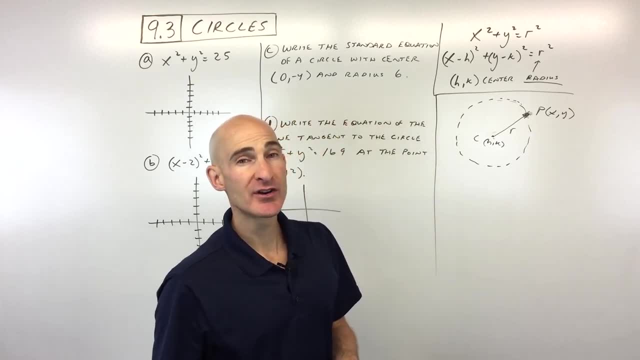 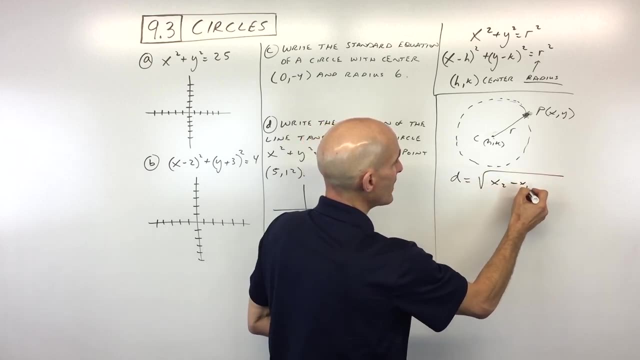 here they're the same distance from the center. So when we think of our distance formula, which we talked about earlier, is the distance is what? It's the square root of x2 minus x1, the quantity squared. plus y2 minus y1, the quantity squared. You add those together. 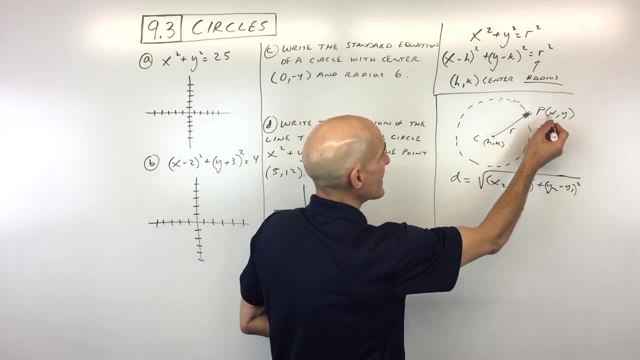 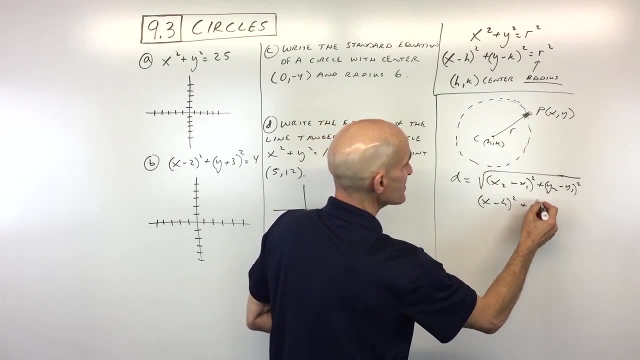 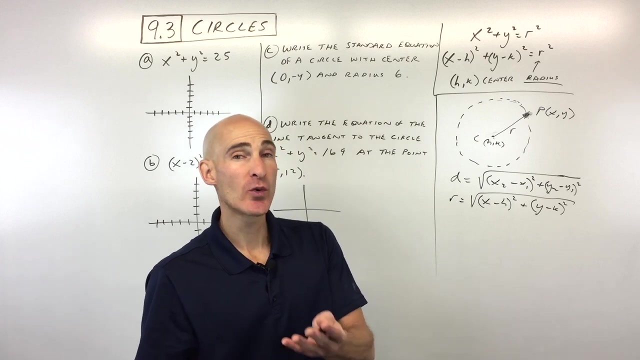 the square root. but in this case we've got x minus h. so we're subtracting the x coordinates squared, and then y minus k. we're subtracting the y coordinates and then squaring, we add those together, we take the square root and that distance is actually the radius. so now, if we square both, 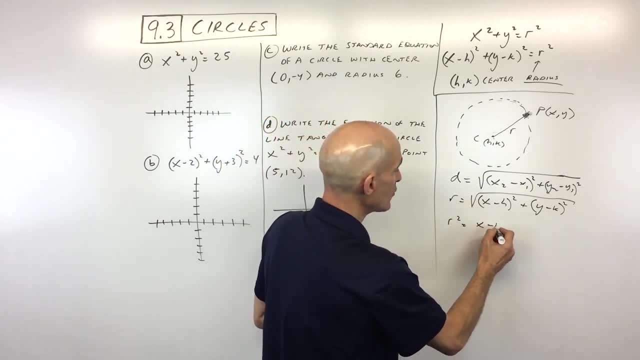 sides of this equation, you can see that you're getting r squared equals x minus h. squared plus y minus k, the quantity squared, because when you square this side, the square and the square root cancel and you square this side to keep it balanced. so you can see that this form right here. 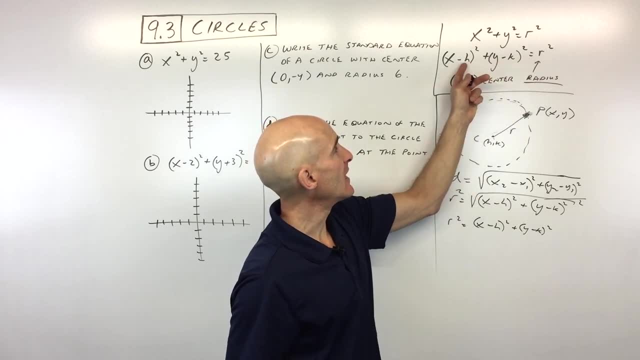 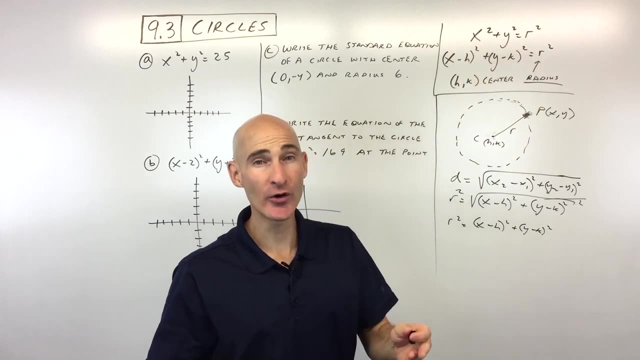 is the same as this form right here. the only difference is is that when hk is at the origin zero zero, then it collapses down to this basic equation: x squared plus y squared equals r squared. okay, so you understand basically where these formulas are coming from. now let's jump into 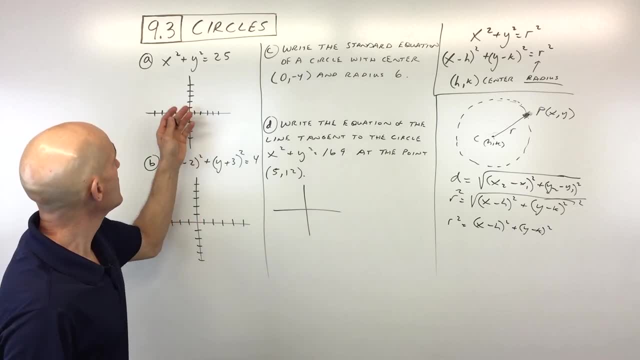 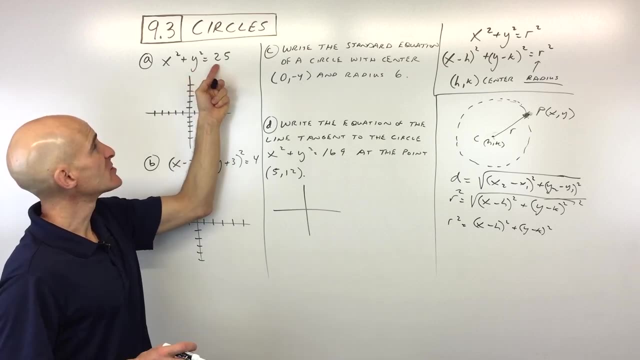 some introductory examples and then i'll have some later that you can practice on your own. the first one: we just want to graph this basic circle here. x squared plus y squared equals 25. so what's the radius of the circle? well, you can see r squared is 25. so that means that r is equal to 5. this hasn't been shifted from the 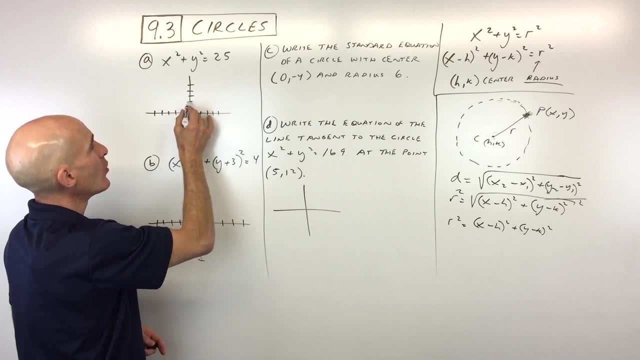 origin. so the center is going to be right here at zero zero. but what we can do is we can go up- five there's a point. down five there's a point on the circle. right five there's a point. and left five there's a point. that just helps us to get a nice you know graph by graphing those four points. 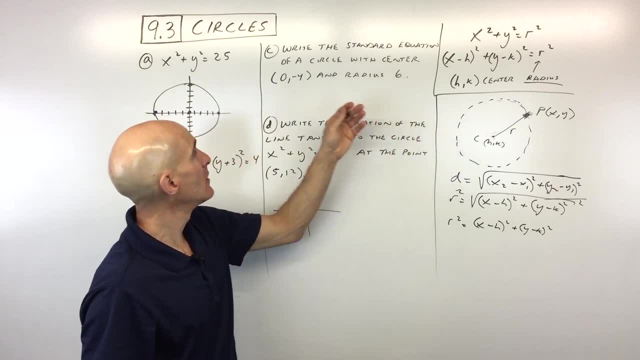 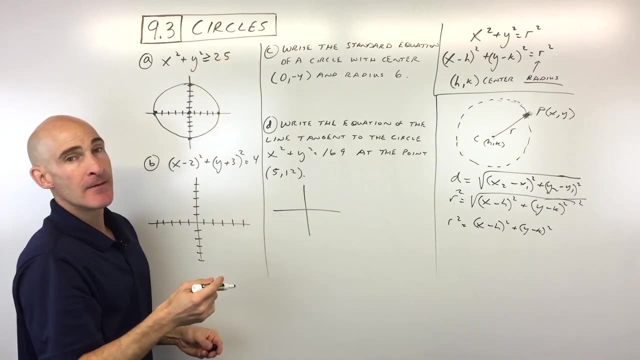 now, one thing that i didn't talk about here, but let me talk about it here. let's say, for example, if we were to make this: instead of equal to 25 greater than, or equal to 25 greater than means that the distance from the center is going to be. 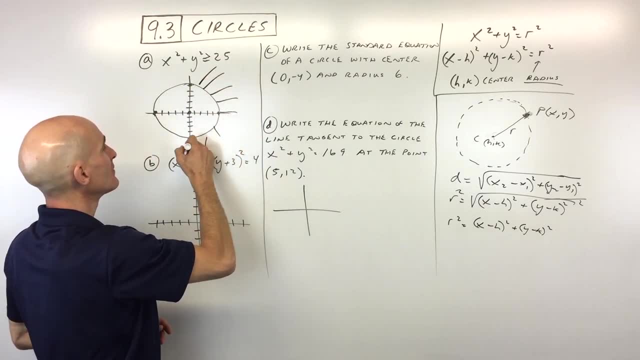 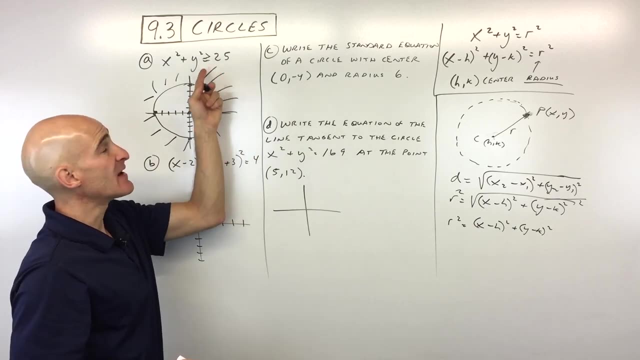 greater or further. so what you would be doing is you'd actually would be shading the outside of the circle if it was less than or equal to, would be shading on the inside if it was less than but not equal to. then it would be like a dashed line, meaning it doesn't include. 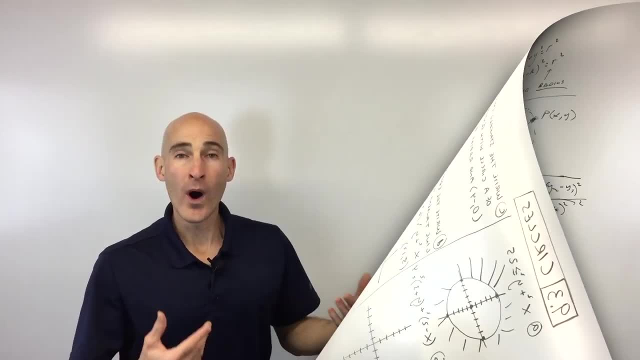 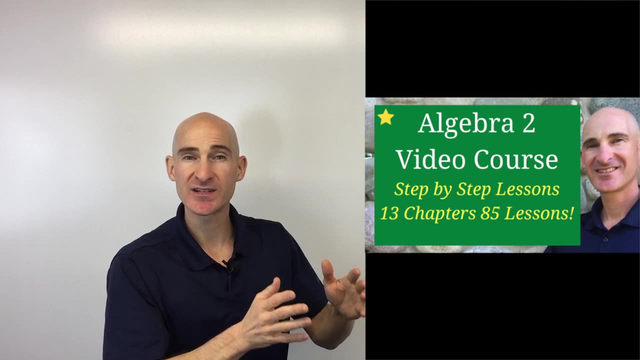 those points on the circle. okay, so that's the basic idea. if you want to learn algebra 2, check out my learn algebra 2 video course for sale, where we go through 85 video lessons that we do step by step by step through algebra 2. we go through the important formulas, concepts as well. 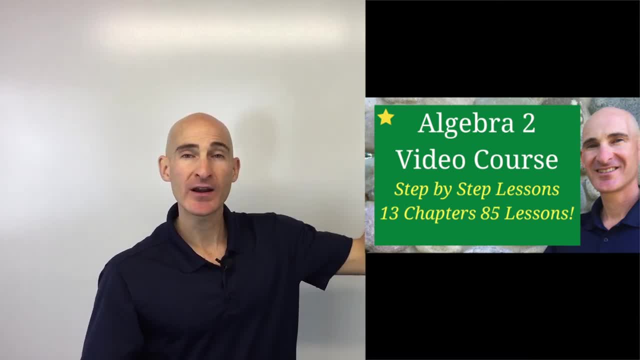 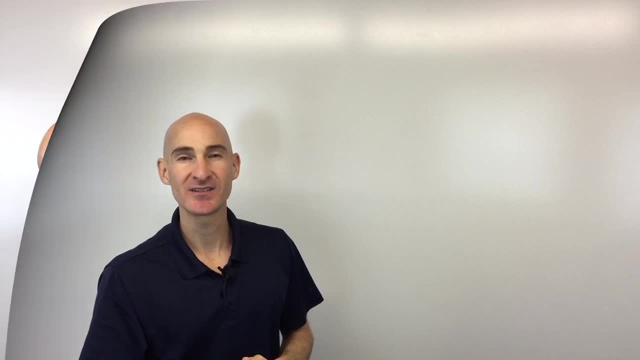 as numerous examples to help you master algebra. 2. click the interactive card or the link in the description below to go over and check out some of the free lessons. otherwise, let's get back into this current lesson. okay, so that's the basic idea. if you wanted to look at it as an inequality, 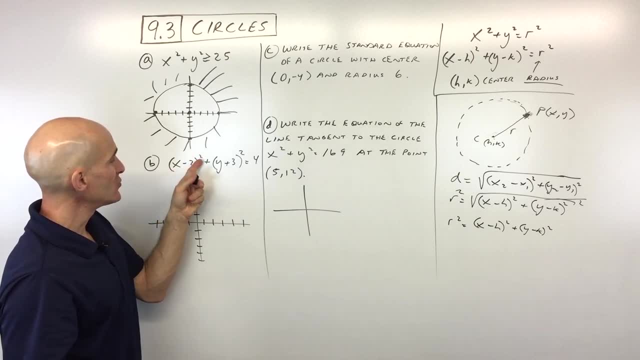 instead of an equation, let's look at letter b now. so we've got x minus 2. the quantity squared plus y plus 3, the quantity squared equals 4.. so here, where's the center? well, the center is going to be negative 2, negative 3. see, these are actually going to be the opposite. it looks like negative 2, but 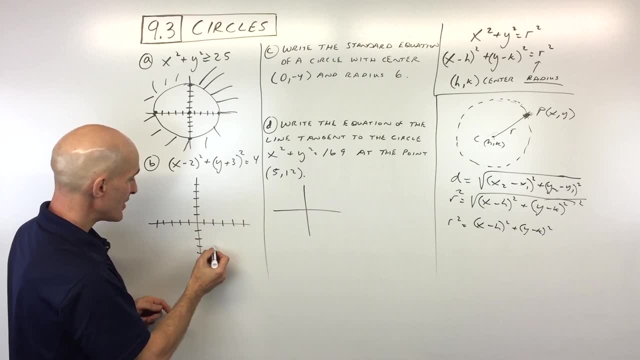 it's actually going to shift right. 2 plus 3. you're actually going to go down 3, so your center is going to be right about there. the radius is 2 because, see, r squared equals 4, so the radius is 2, so we're. 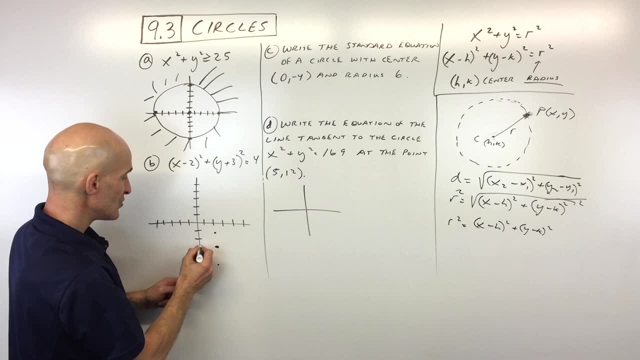 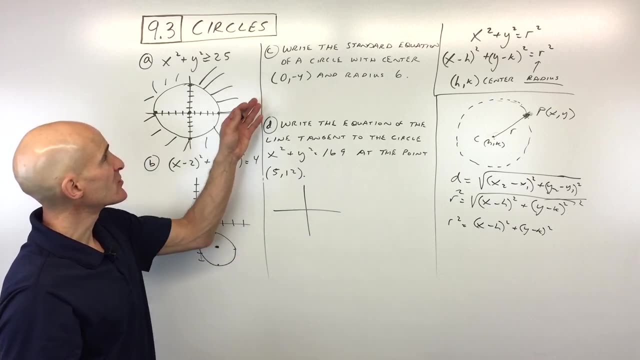 going to go up 2, down 2, left, 2, right, 2, and that's just to give us a couple of points so that we can get a better, you know, sketch of our circle. okay, let's look at letter c now. it says: write the: 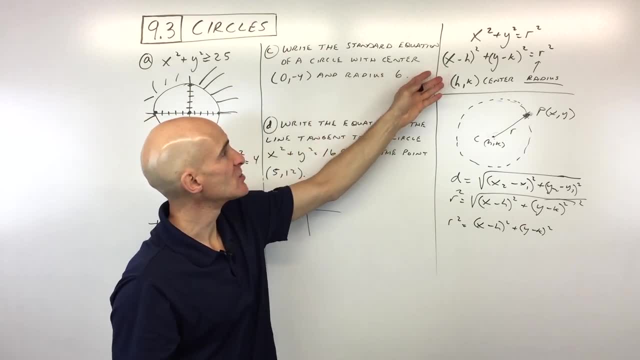 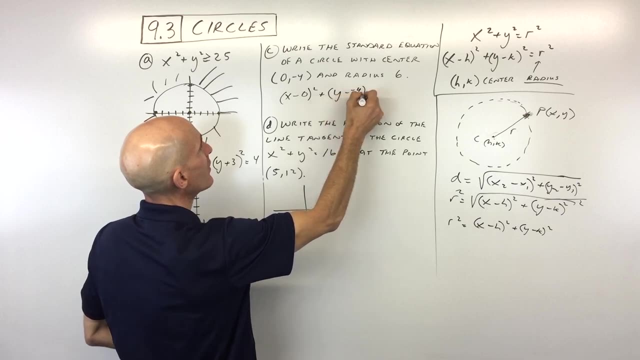 equation of the line that's tangent to where q equals and radius of 6.. so now we're having to write the equation, so we're just working backwards here. we're saying: x minus 0 squared plus y minus negative, 4 squared equals 6 squared, which is 36.. so if we simplify, we just get x squared plus y. 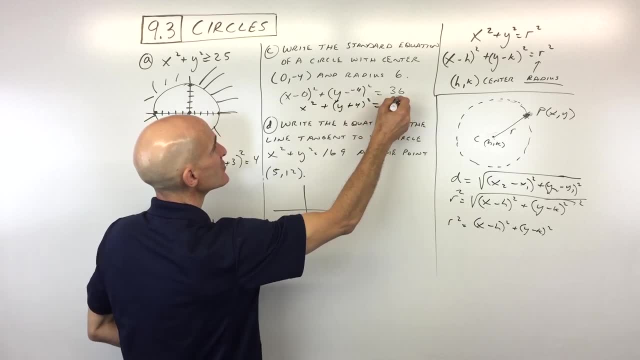 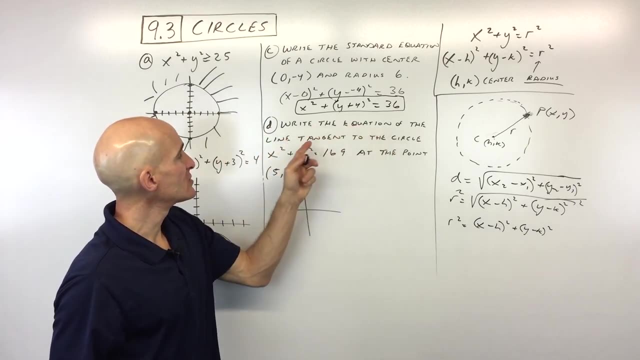 plus 4 squared, since the two negatives here cancel and give you a positive, equals 36, and that's our standard form of the equation of a circle. okay, now letter d. it says: write the equation of the line that's tangent to where q is a square, be at least between the non- ticks and a non- quiser, so an x and 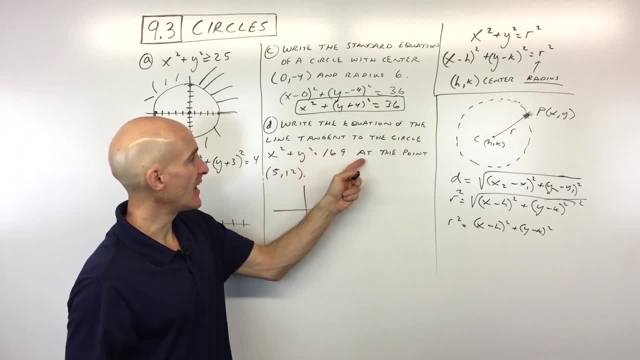 q, that's negative, plus 3 and y are going to be, with the smallest negative, 2.. now let's go and see 3 pa to the circle: x squared plus y squared equals 169, at the point 512.. Okay, so it helps to draw. 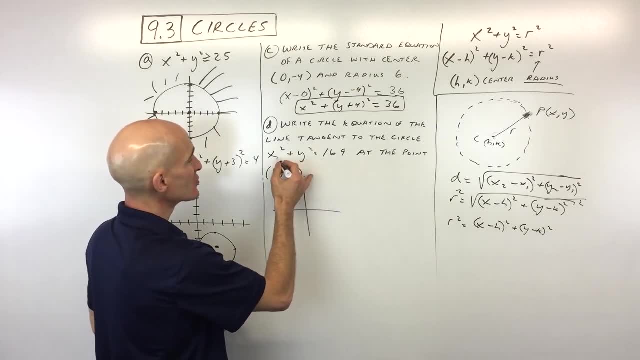 a sketch when you do these types of problems. But you can see that this is a circle that's centered at the origin. The radius is the square root of 169, which is 13.. So if I go up, 13,, down 13,, right 13,, left, 13.. Okay, we've got some points. There's our circle. It's tangent to the circle at 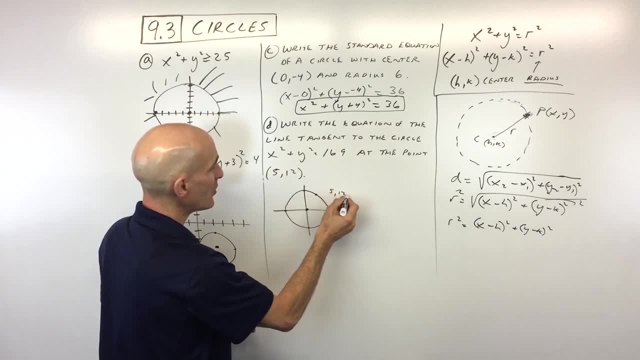 the point 512, which is right about there, 512.. Now if you make this into a triangle, see how I went right 5 and up 12?. When you do the Pythagorean theorem you'll see that that hypotenuse that. 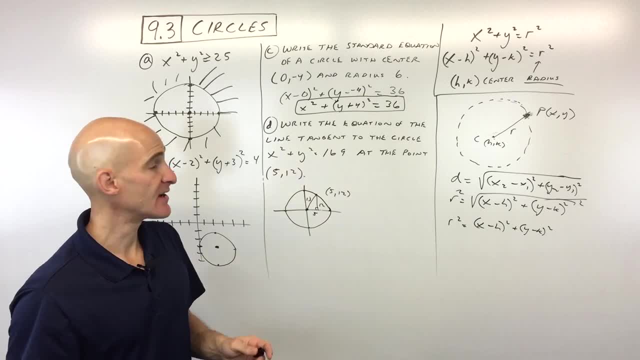 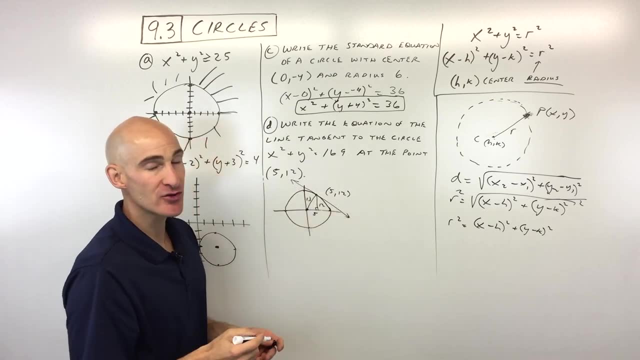 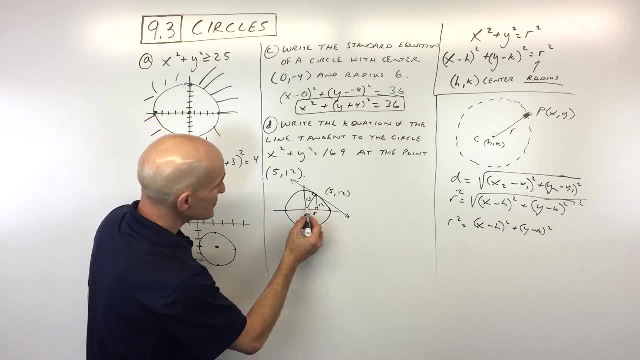 perpendicular. Okay, so what we want to do is we want to find the slope of this line, which is going to be, let's see, rise 12, run 5.. So that means the slope is going to be 12 fifths, But the 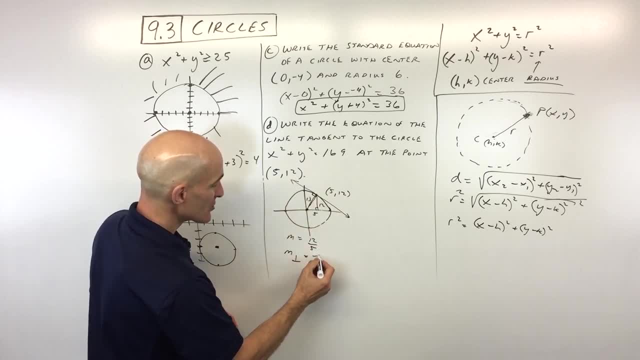 perpendicular line is actually going to have the opposite reciprocal slopes of negative 512.. So that's the slope of this line And we know it goes to the point 5, 12.. So if we put it all together into an equation using our point slope form, we get: y minus 12 equals the slope which is negative 512. 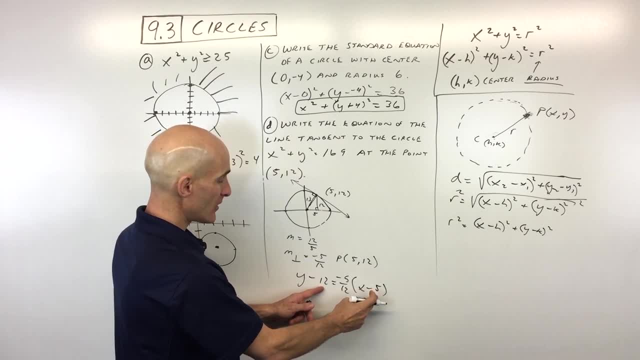 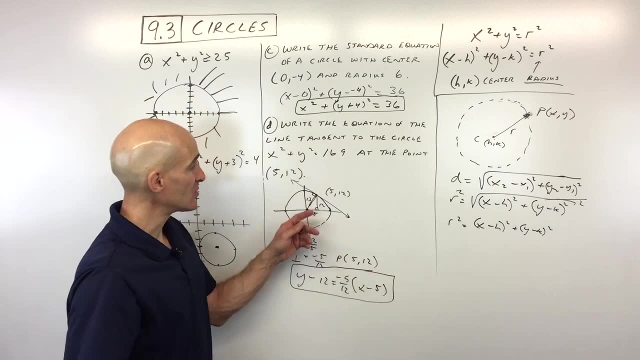 x minus 5.. So there's our point x1, y1.. There's our slope negative 512.. And that's the equation of your tangent line to the circle at the point 5, 12.. Now, if you wanted to, you could distribute. 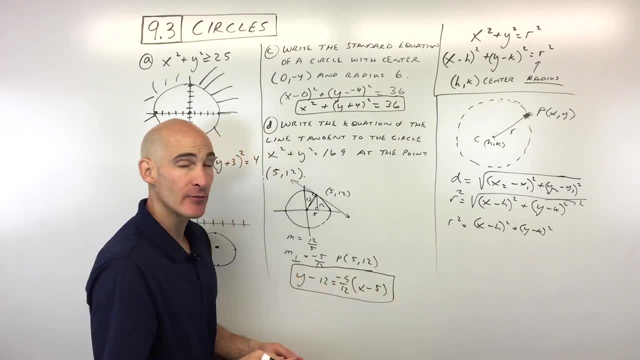 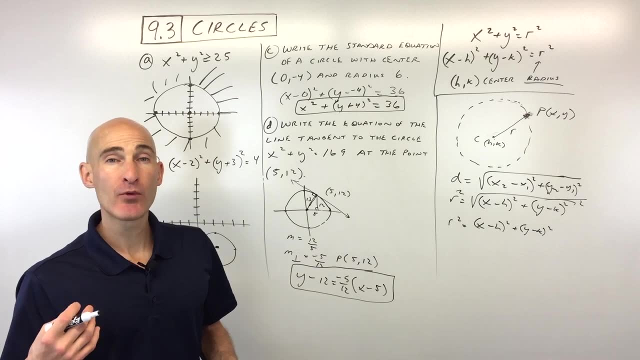 this negative 512.. So you could add the 12 over here to get the y by itself and put it into the y equals mx plus b form, the slope intercept form. But for right now let's just leave it like that. Okay, so let me erase the whiteboard. I've got some problems that you can practice on your own. 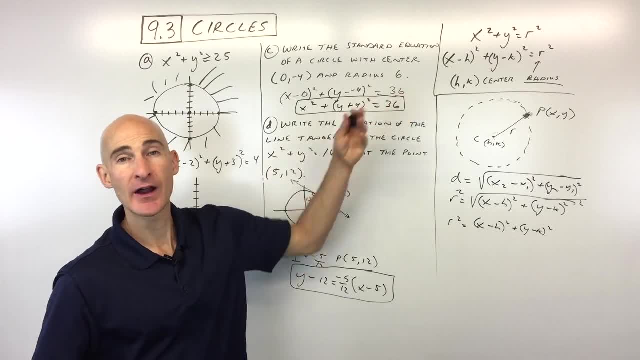 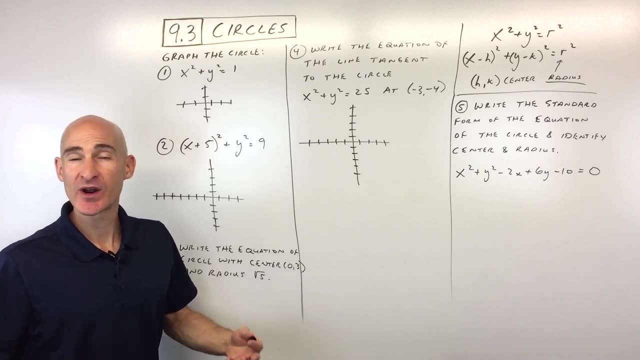 to get some more experience with the standard form of the equation of a circle, How to graph circles, how to write equations, etc. So we'll jump into those next. Okay, here's your opportunity to practice graphing these circles, writing equations, etc. So let's. 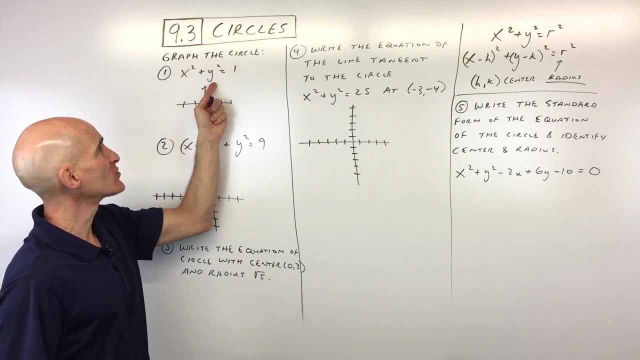 start with number one. How would you graph this circle? x squared plus y squared equals 1.. So we're just starting off basic. We'll get more challenging as we go through these problems. But what do you think? How would you graph that circle? Go ahead and pause the video, do it? 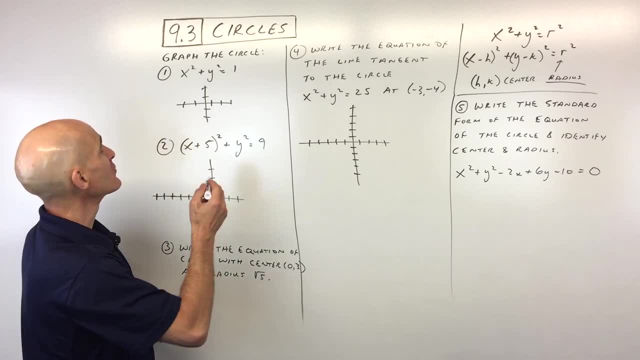 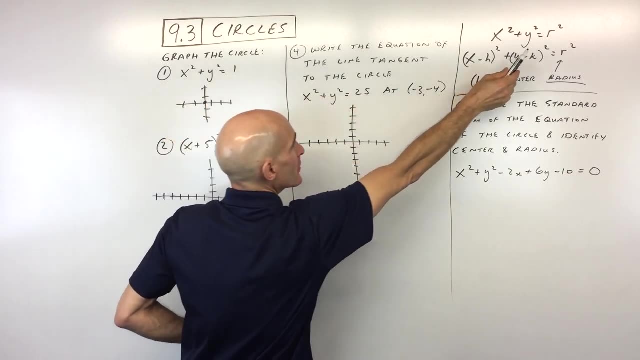 and we'll go over it together. So this one, you can see it's not been shifted from the origin, So the center is going to be right here at 0, 0.. Now, remember, this is the radius squared right. So if you set r squared equal to 1, and you take the square root, 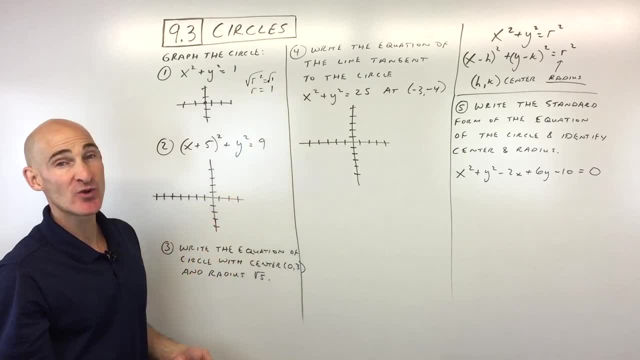 of both sides, you get still. you get 1, right, Because 1 times 1 is 1.. So here the radius is really just 1.. So you're just going up 1, down 1, right 1, left 1.. So it's just a circle with. 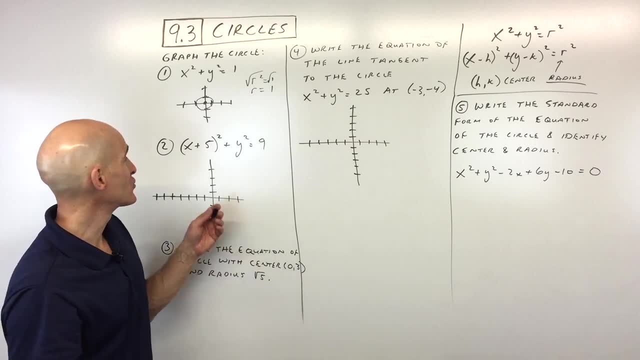 radius 1, centered at the origin. Pretty easy. Let's go to number two, a little bit more challenging. How would you do this? one x plus 5, the quantity squared plus y squared equals 9.. How would you graph that one? Well, you can see that the center is going to be at 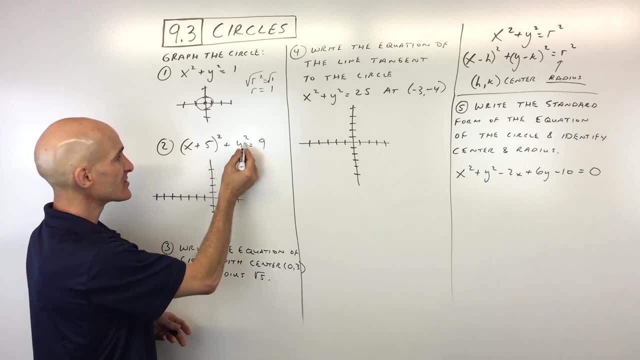 the opposite of 5.. So negative 5.. And here it's not shifting up or down, So it's going to be negative 5, comma 0.. So that's our center: 1,, 2,, 3,, 4, 5, to the left. negative 5, comma 0.. And then r squared. 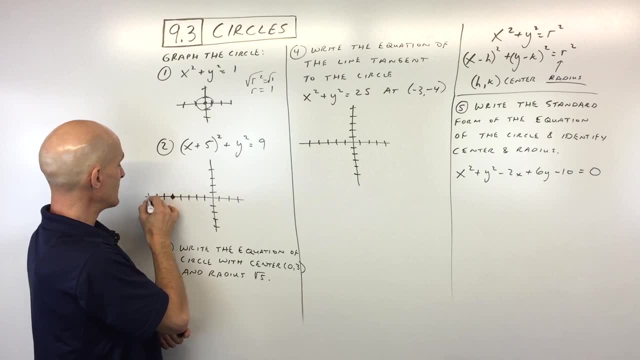 equals 9.. So we can see that the radius is 3.. So if we go, let's see left 3, right 3, up 3, and down 3, okay, you get a few points to get a nice sketch of your circle And you got it. 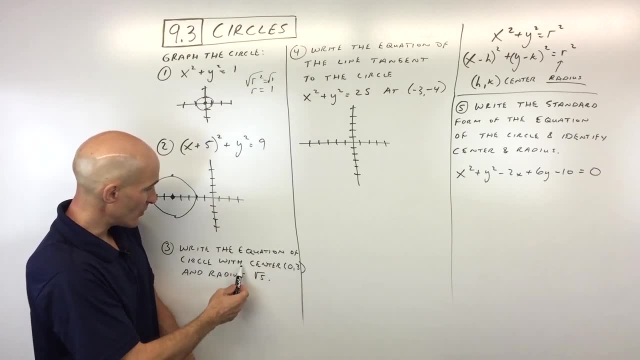 Okay, let's look at number three. Now, here it says: write the equation of the circle with 0,, 3 and radius square root of 5.. Okay, so how would you do that? one See if you can pause the. 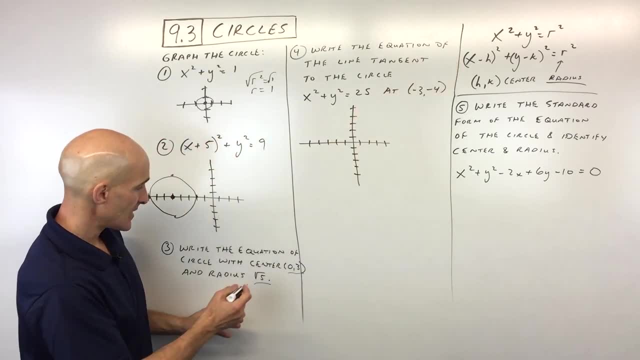 video We're going to use these formulas over here. You can see that the center is 0, 3.. So we have x minus 0, squared, plus y minus 3, the quantity squared equals the radius, which is square root of 5, squared because, remember, it's r squared. Well, the square and the square root. 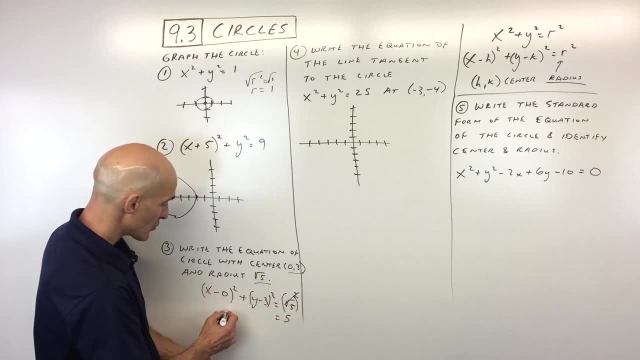 here they cancel one another out. You just get 5.. x minus 0 is just going to be x. So we have x squared plus y minus 3. squared squared is equal to 5.. That's the standard form of the equation of a circle. Okay, so let's go to. 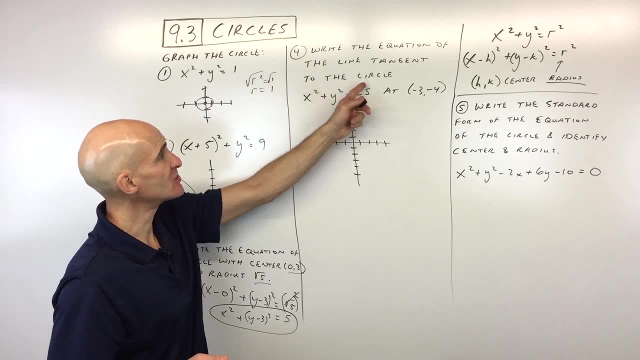 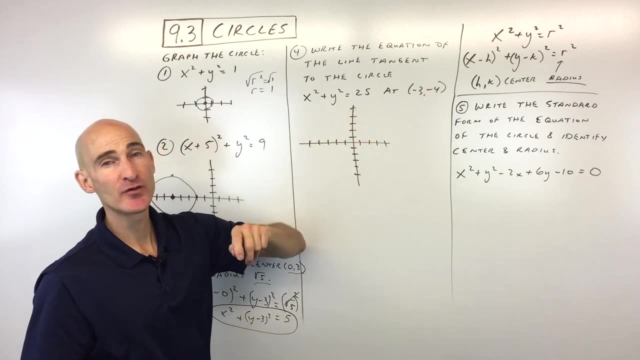 number four. now We've got write the equation of the line that's tangent to the circle. at the circle, x squared plus y squared equals 25.. This is the circle we're working with And it's tangent at the point negative 3, negative 4.. So how would you do that one? Well, if we graph this circle, 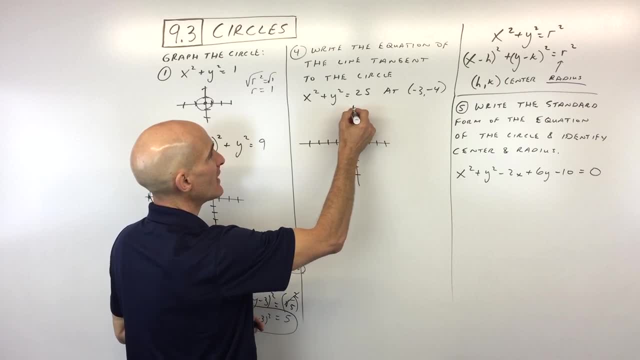 you can see, it's centered at the origin. The radius is 5.. So if we go up 5, down 5, right 5, and left 5, we've got a few points on our circle, Okay. and if we go, let's see left 3 and down 4,. 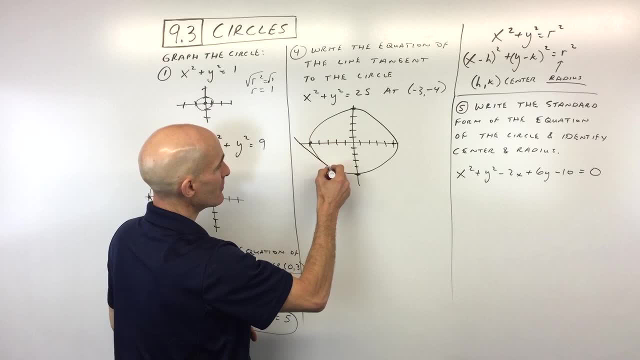 there is the point that the tangent line is just going to barely touch the circle. at that point, negative 3,, negative 4.. Now if you draw a radius to that point of tangency, okay, where it's tangent, the radius and the tangent line are going to be perpendicular. So if we look at the slope of this, 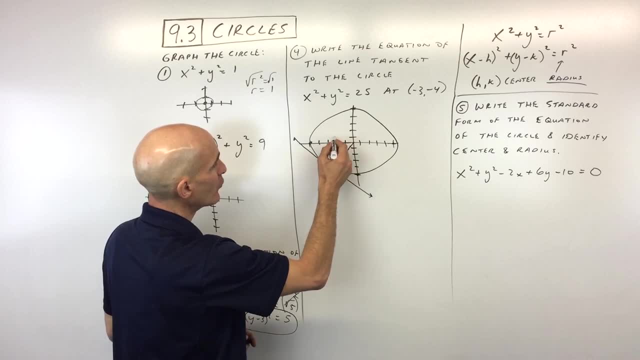 line right here. see how we're going left 3 and down 4, left 3 and down 4.. But the slope, remember the slope is the, the rise over the run. So we're going down 4, that's negative. We're going left 3, that's negative. The two negatives cancel. 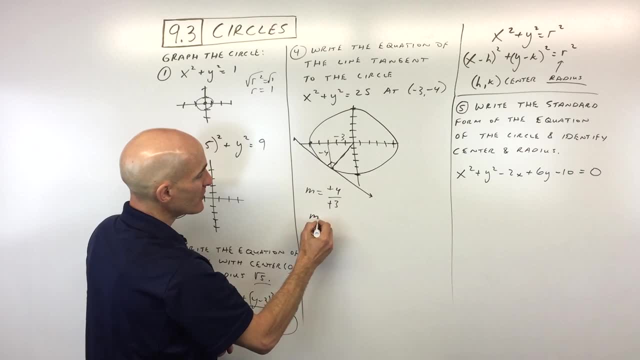 gives you a positive 4 thirds. But when you find the slope that's perpendicular, it's going to be the opposite, reciprocal. So you're going to change a sign to the opposite and you're going to flip the fraction. So the slope here is going to be negative 3 fourths and it goes through the point: negative 3, negative 4.. 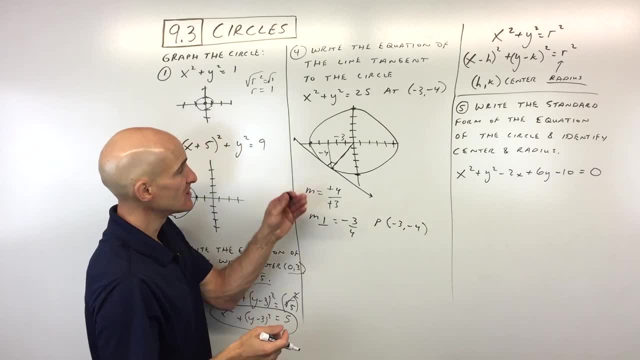 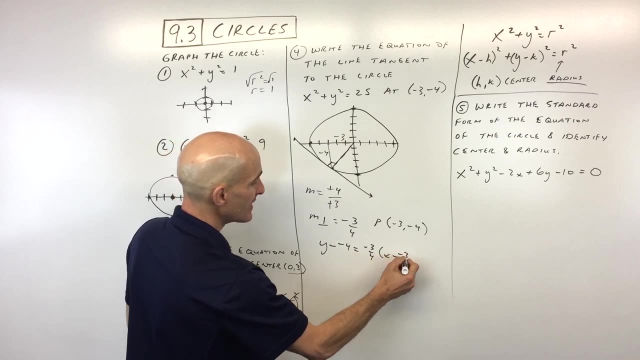 So if you have the slope and you have a point point, slope form is going to be the easiest way to start writing your equation. So it's going to be 1, 2, 3, 4.. So y minus negative 4 equals the slope times x minus negative 3.. 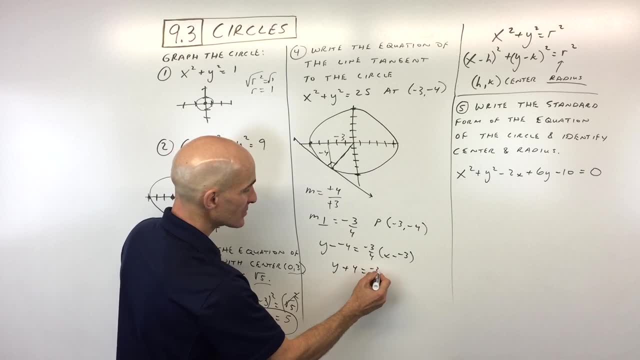 And you can condense this down a little bit. The two negatives are going to give you a positive, And then same thing here. If you want, you can distribute the negative 4th and subtract 4 to get y by itself. to put it in the slope. 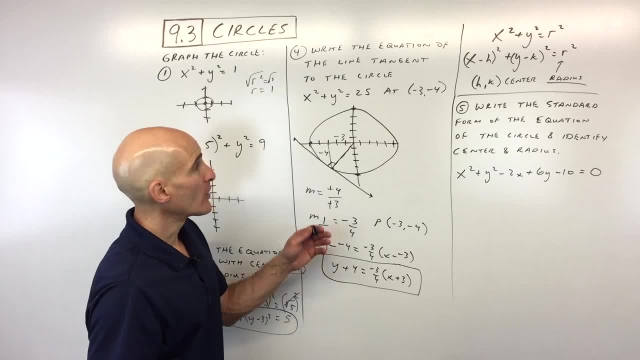 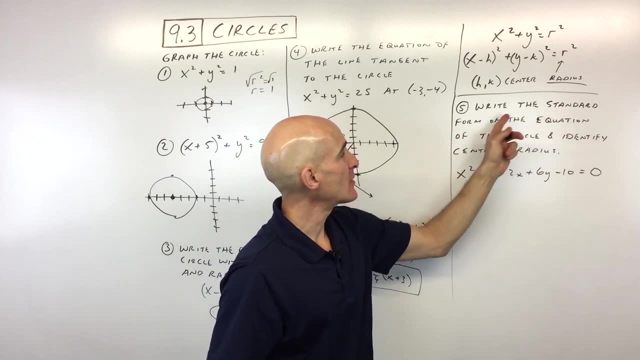 intercept form. But that's pretty good for right now. Okay, last question: See if you can do this one. This one we didn't talk about in the introductory examples, but I think you can figure it out. It says: write the standard form of the equation of the circle and identify the center and. 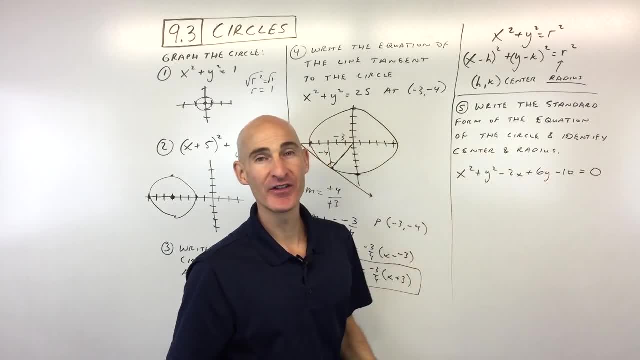 the radius. Now notice, they're just giving us all these terms here and it's kind of a little kind of complex or messy, I guess you could say. But what we need to do- I'll give you a hint- is: you want to complete the square And we're trying to get it looking like the standard form. 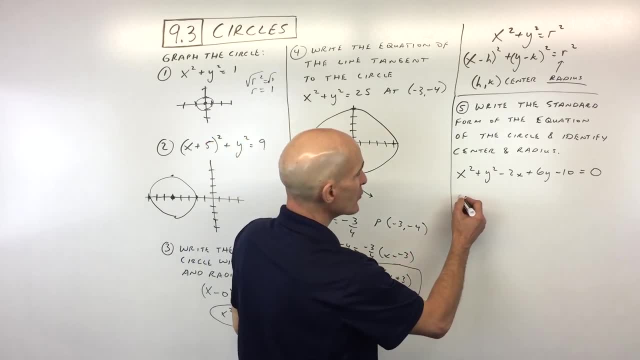 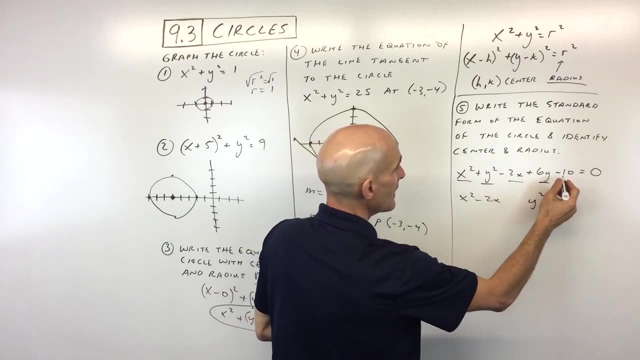 of the equation of a circle. So what I would do here is: I would group the x's together, See x squared, and negative 2x. I would group the y's together, y squared, and 6y The negative 10,. 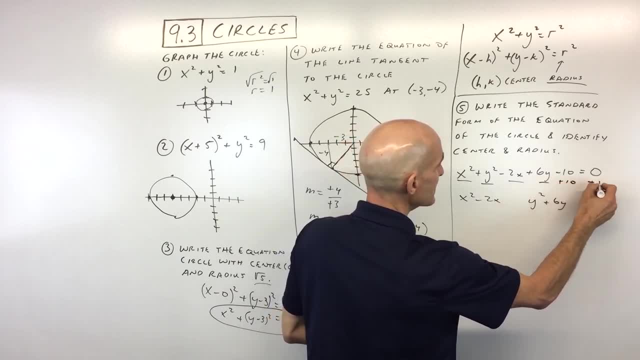 I'm just going to add to the other side. It's like it's going to be: if I add 10 here, I add 10 here. right Now we're going to complete the square. So we take half of negative 2, which is negative 1.. 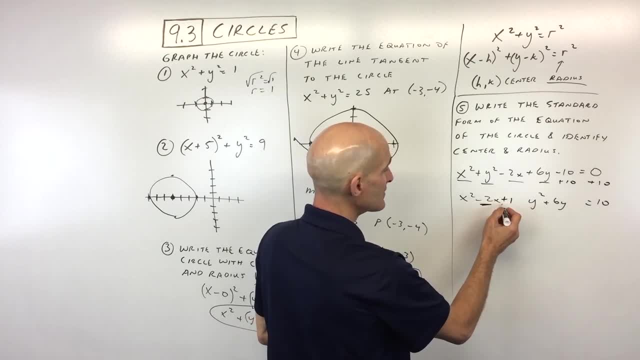 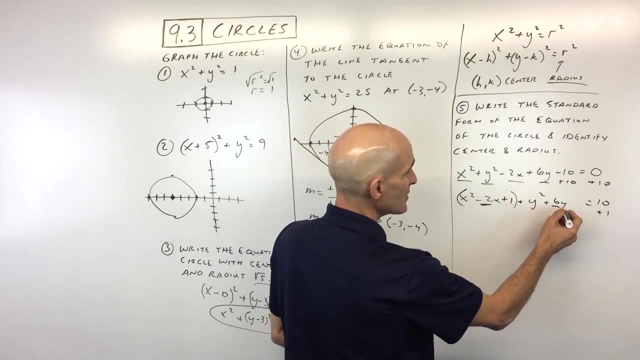 If we square it, that's going to be positive 1.. But if I add 1 to the left side of the equation, I have to add 1 to the right to keep it balanced. right And over here I have, half of 6 is 3. 3. 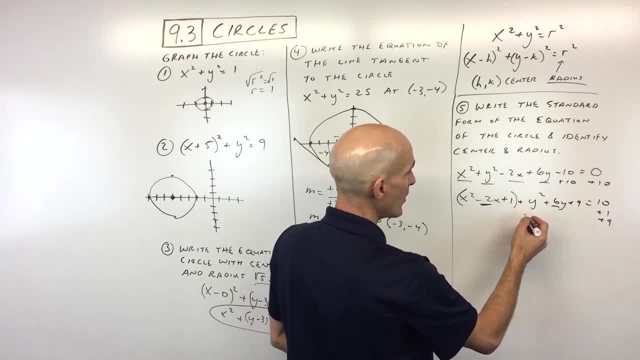 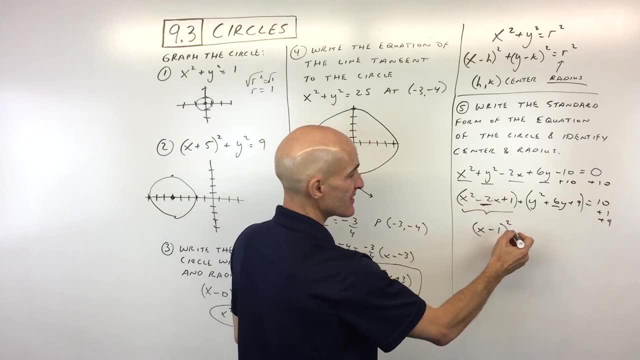 squared is 9.. But if I add 9 to this side, I have to add 9 to the other side as well. So now you can see that we've got this as a perfect square. x minus 1 squared represents that there, And if we 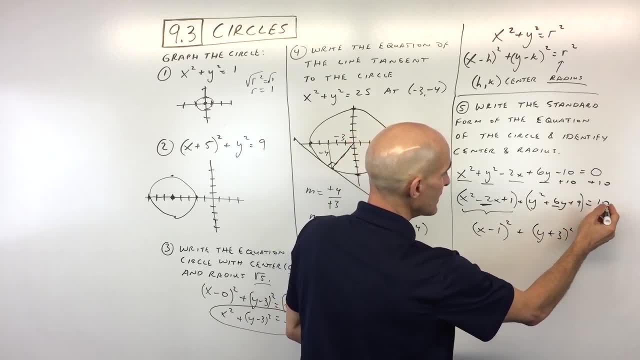 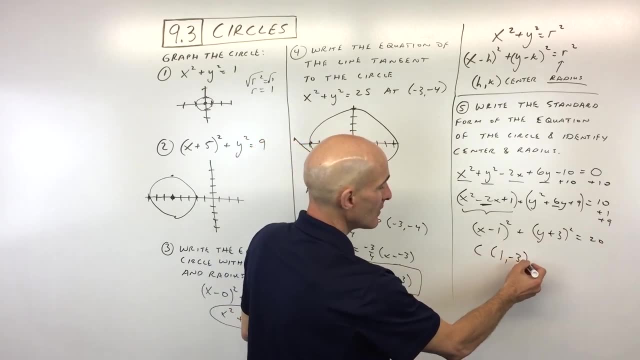 factor this, we get y plus 3.. squared, And here we get 20.. So now what you can see is that the center is going to be at 1 comma negative 3. And the radius is actually going to be the square root of 20, which you 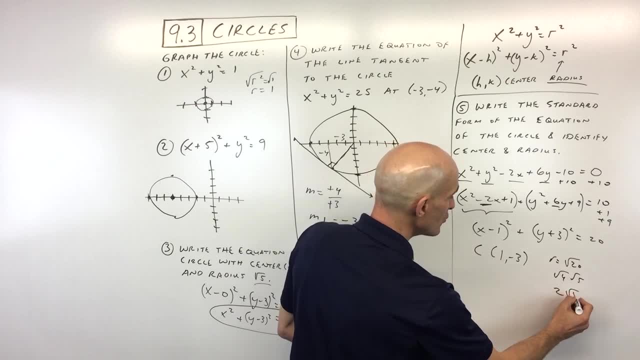 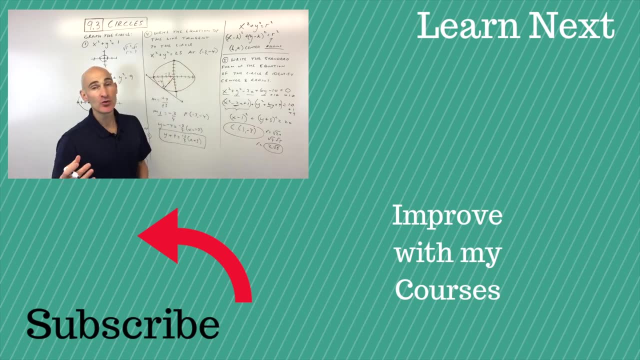 can simplify, That's 4 times 5.. Square root of 4 is 2.. So the radius is going to be 2 square root of 5.. So center 1 negative 3 and radius 2 square root of 5.. So great job If you need to review. 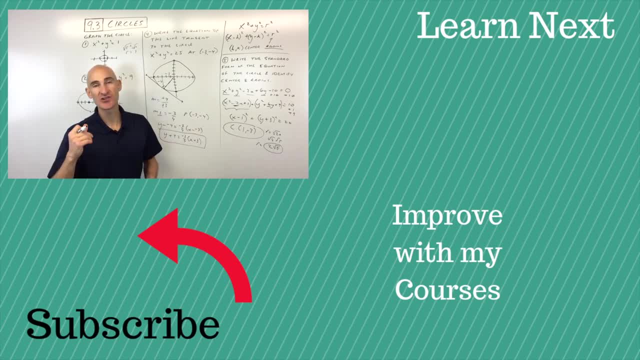 this lesson. go ahead and do that covering all about circles, Otherwise I'll see you in the next lesson. Thank you for watching.